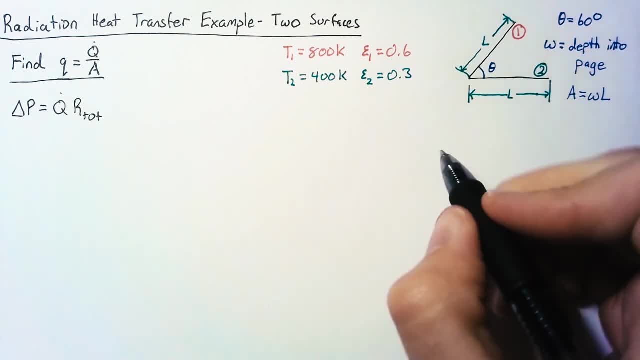 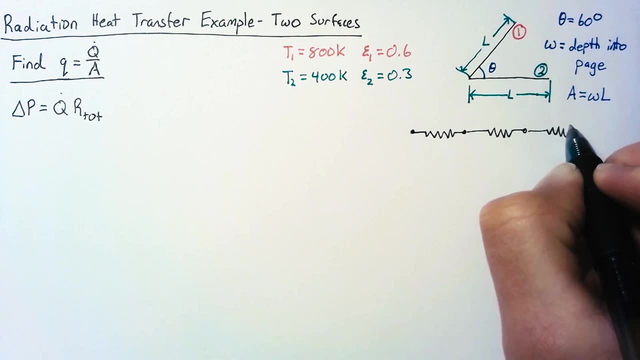 So the picture that we'll draw as a resistive circuit is simply three resistors connecting our two surfaces: On the left- here we're going to have the blackbody radiation of surface one, And on the right, we're going to have the blackbody radiation of surface two. 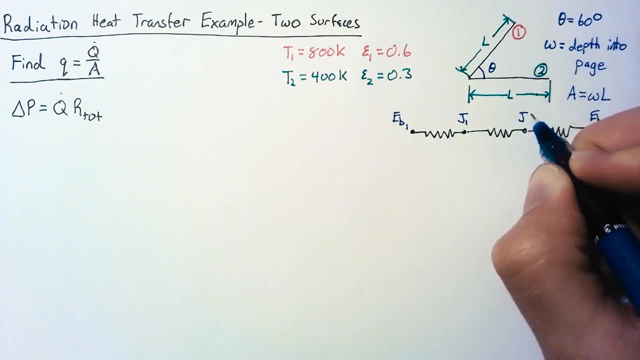 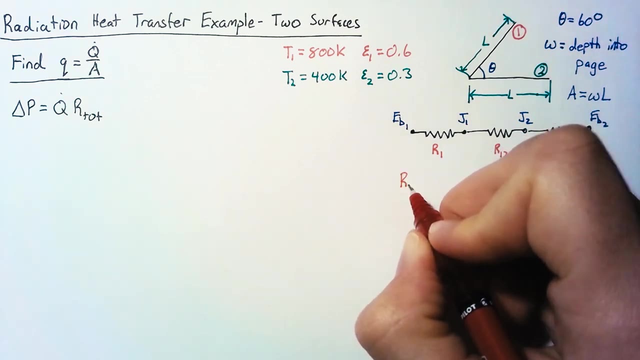 And then these two points in the middle are just the radiosities of our two surfaces. Now, in previous videos we called these resistors R1, R2, and R3.. R1 and R2 are our surface resistances And we can write R1 as one minus epsilon, one over epsilon one a. 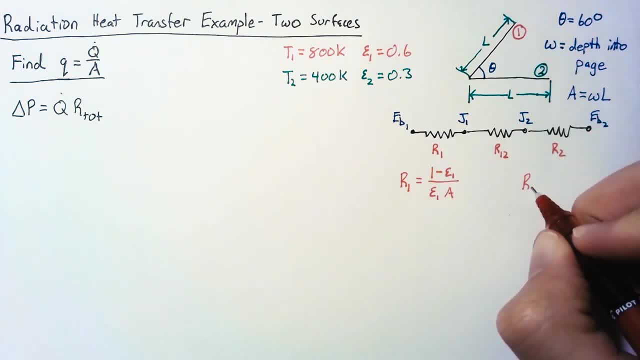 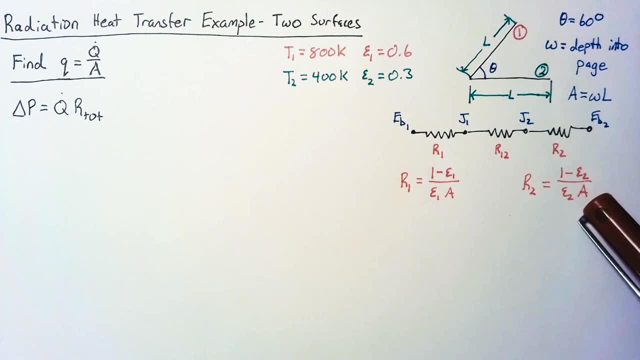 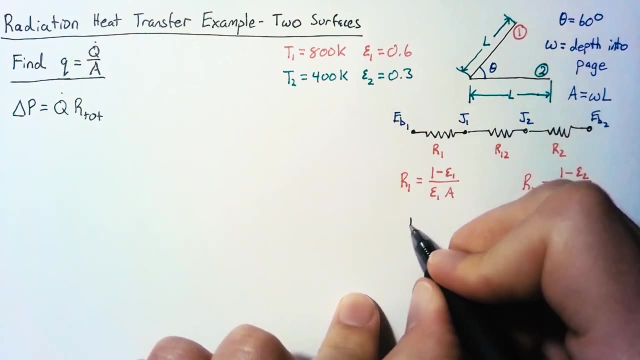 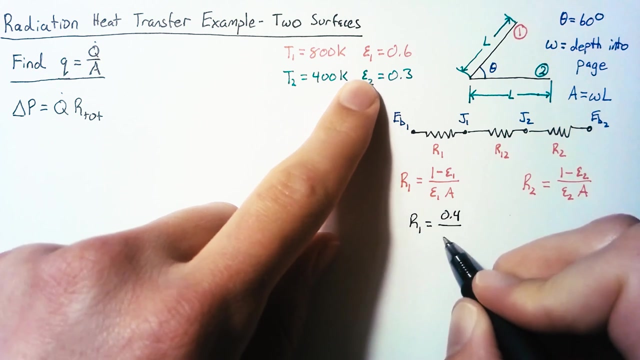 Likewise, R2 will be one minus epsilon two over epsilon two a, And I'm able to use this general a since our surfaces have the exact same area. Now we can go and plug in values for epsilon one here And we can say that R1 is going to be one minus 0.6, or 0.4 divided by 0.6, multiplied by one over a. 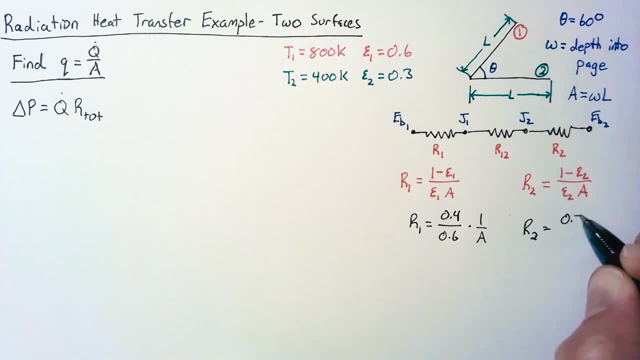 Doing the same thing for R2 gets us 0.7 divided by 0.3, multiplied by one over a. This middle resistor is our space resistance, And that's just equal to one over a multiplied by the view factor. So here we need to go look up what the view factor is. 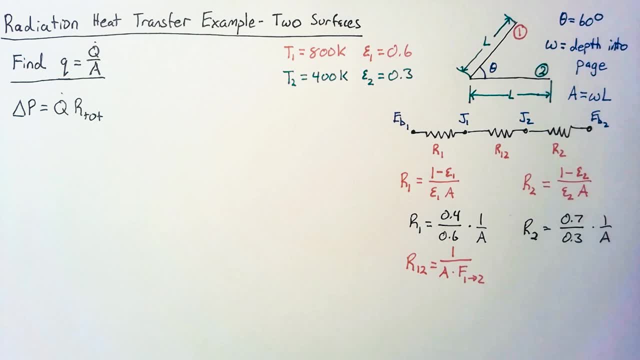 And for this geometry our view factor is equal to one minus sine of one half times theta. So plugging in theta here, we end up with sine of 30. Sine of 30 is one half, and so we end up with. 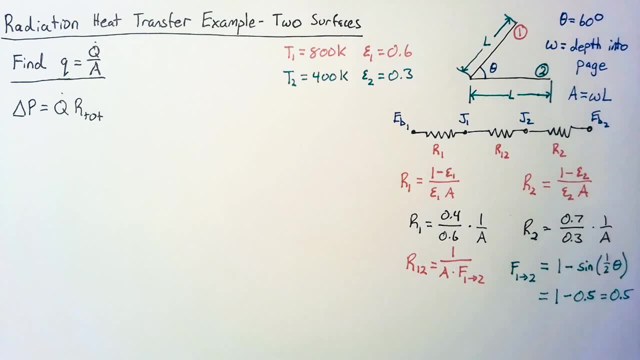 just a view factor of zero point five, 5.. So plugging the 0.5 in, we end up with a space resistance R12, which is equal to 1 over 0.5, or 2 times 1 over A. So putting that all together, our total resistance is going to: 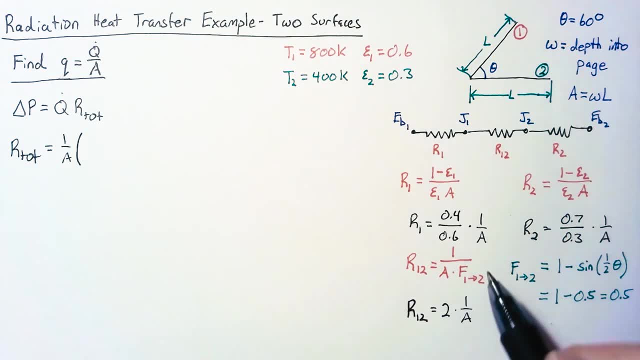 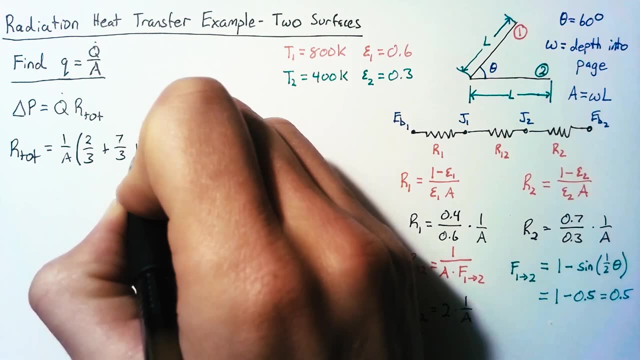 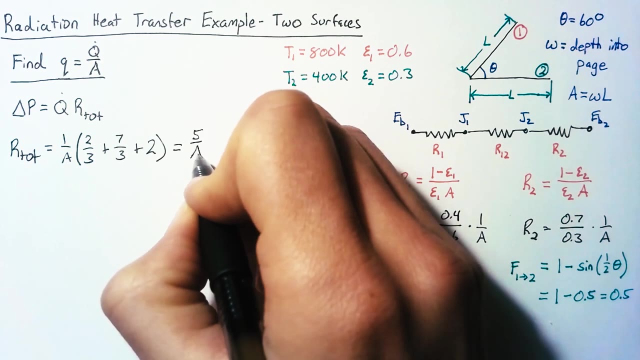 be equal to 1 over A, multiplied by 0.4 over 0.6, or just 2 thirds plus 7 thirds plus 2.. So simplifying that we just end up with a total resistance of 5 divided by A. So next we need: 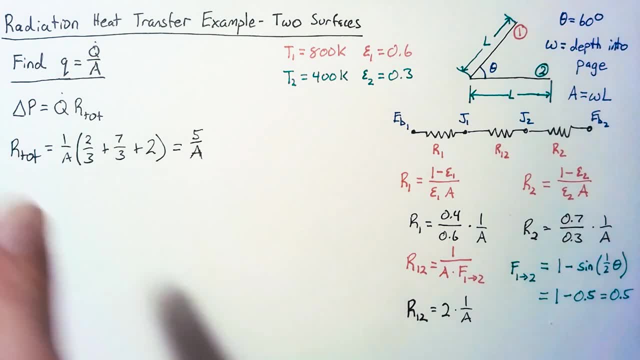 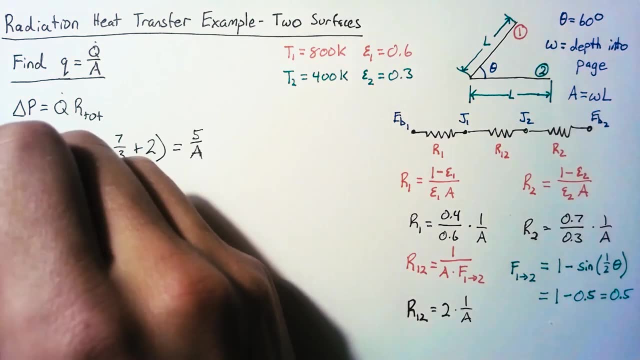 to find this delta P, the change in potential. And the change in potential is just going to be the difference. in these EB terms, Our blackbody radiation from surface 1 is going to be sigma multiplied by T1 to the 4th. 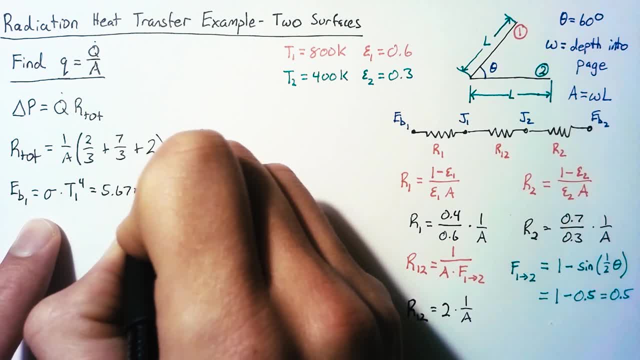 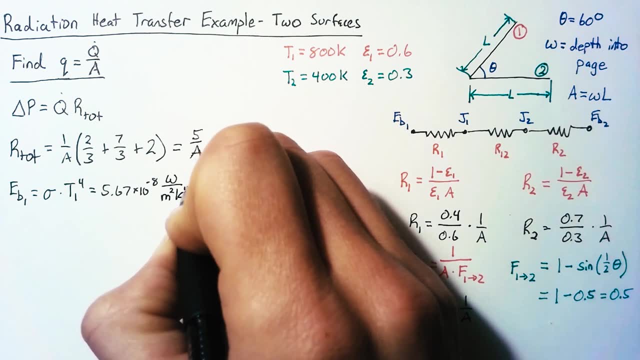 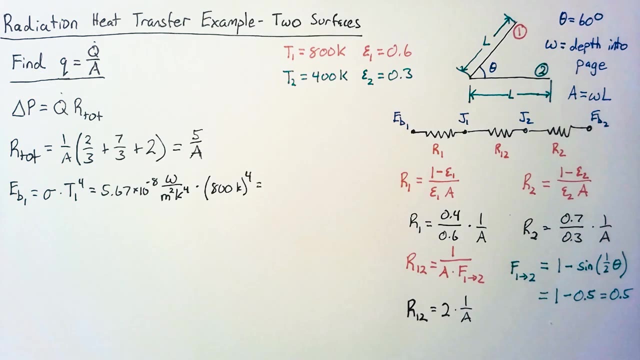 The sigma is 5.67 times 10 to the negative 8, and that has units of watts per meter squared Kelvin to the 4th, and that'll be multiplied by 800 Kelvin to the 4th. So plugging that in, 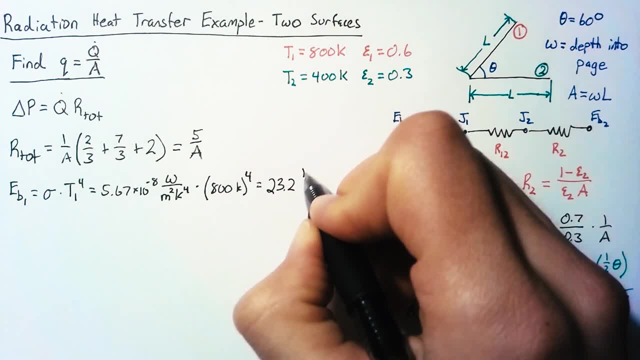 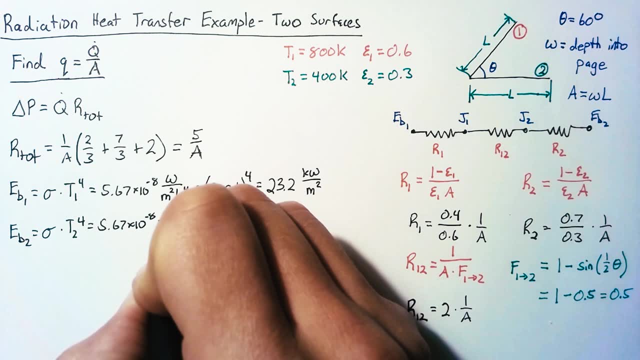 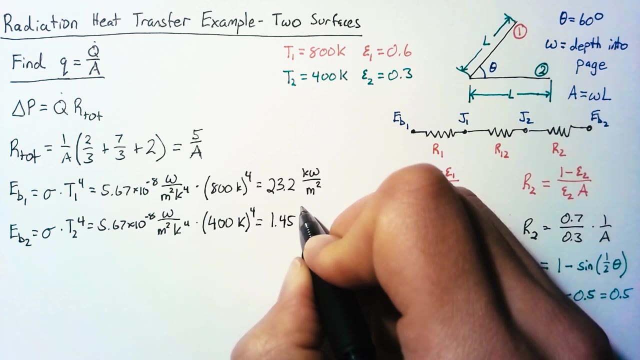 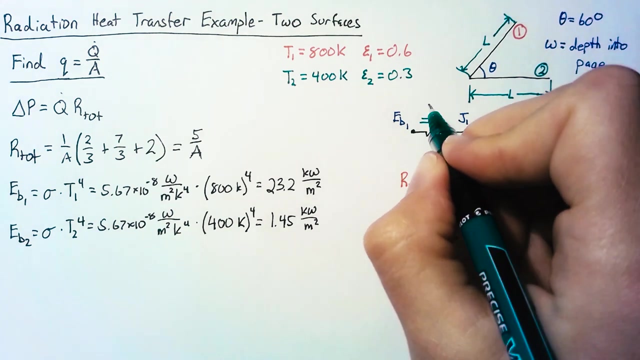 we end up with 23.2 Kelvin, So that's 4.37 kW per meter squared. EB2 will do much the same way And that'll end up as 1.45 kW per meter squared. So, defining our Q-dot as moving from left to right, We can say that our delta P is equal to. EB1 minus EB2.. And that'll be equal to E1 minus E2.. So we're going to end up with R12 times T1, multiplied by 0.4 over 0.6.. So we end up with 1.47. 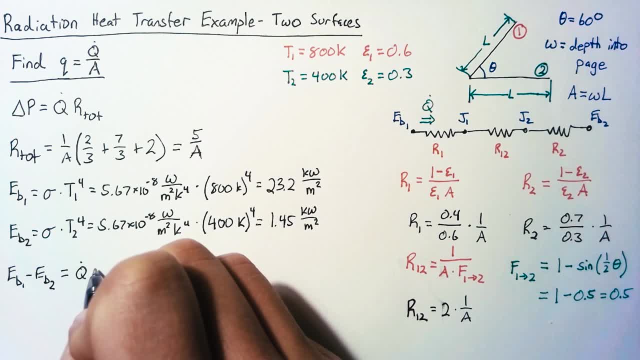 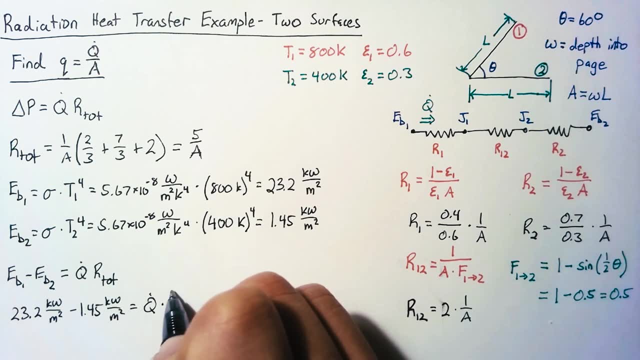 kilo watts per meter squared, EB1 to the 4th to Q dot, multiplied by our total resistance, So plugging things in, we can see that our heat flux just naturally falls out here. So that's the Q that we're looking for, And so we have this number. 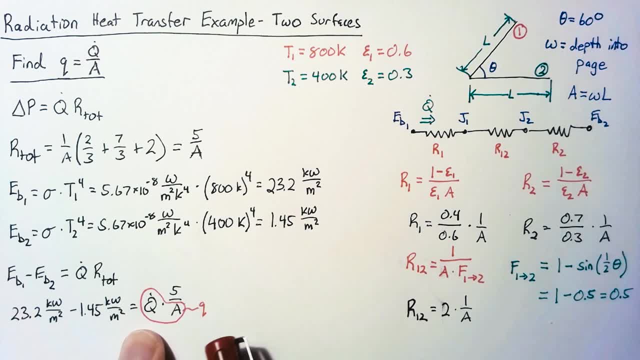 on the left is going to be equal to 5 times Q, So all that's left is to plug and chug and we end up with. Q is equal to 4.35 kilowatts per meter squared, And that is how we handle radiation heat transfer.